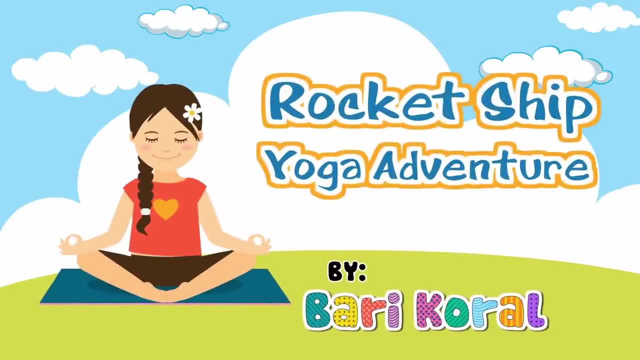 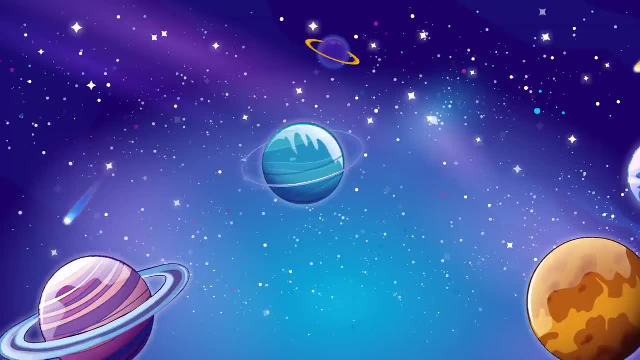 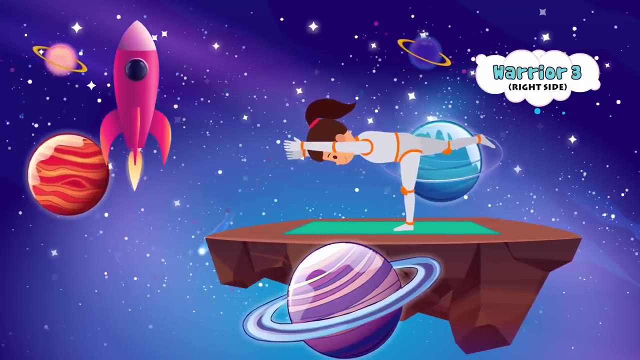 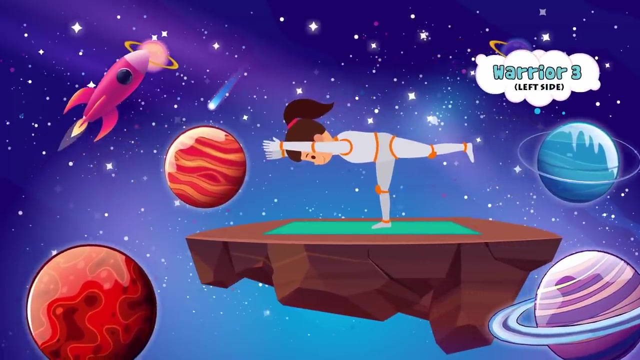 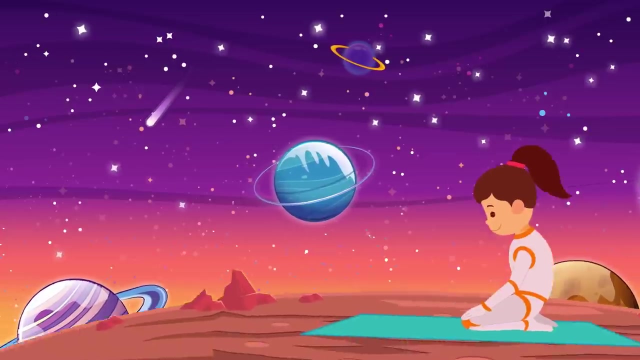 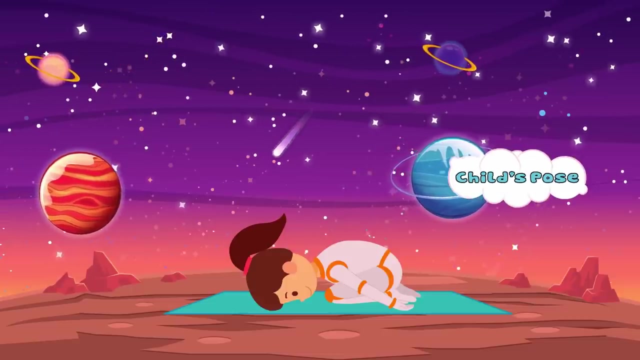 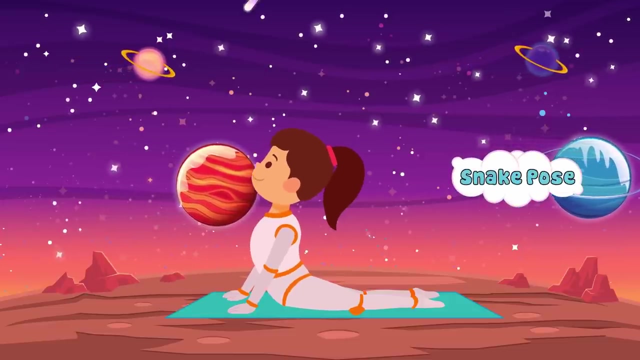 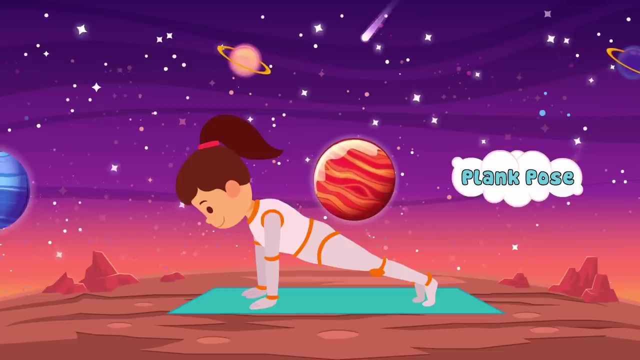 I like to take a rocket ship to the moon. Here's the part where we go zoom. We fly out out to outer space. Fly out out to outer space. I wanted to be a pilot ever since I was a child. I would gaze up at the stars looking for Mars. Fly a big rocket, go far into orbit. 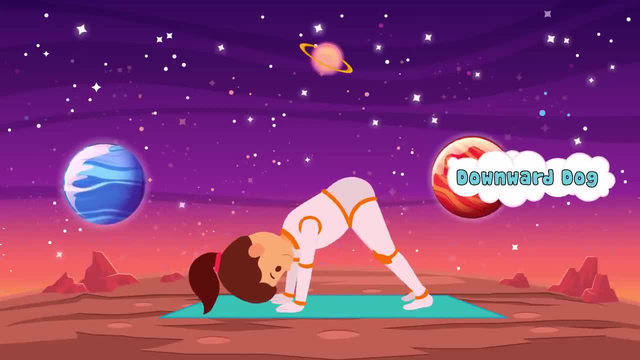 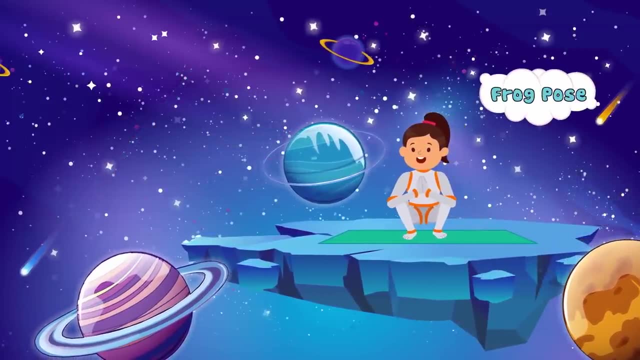 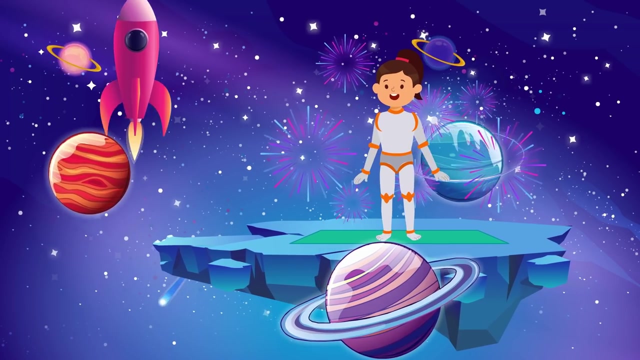 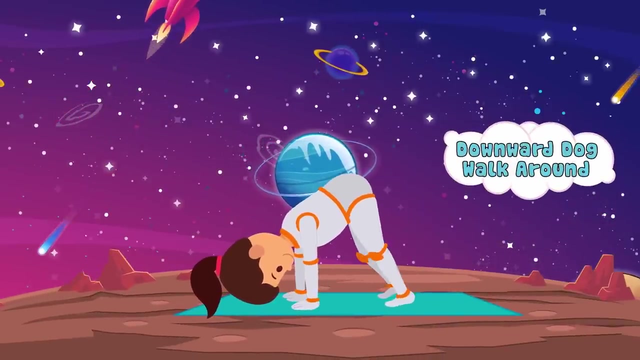 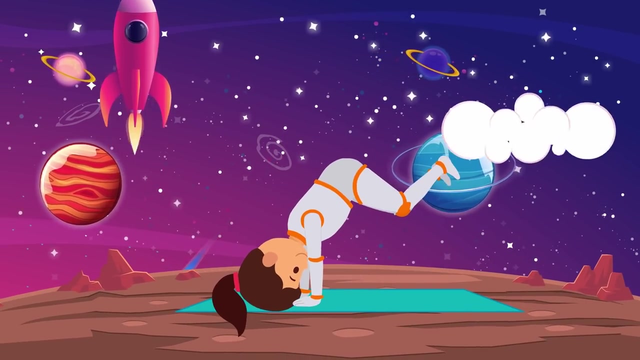 Blast into space to see what awaits. Oh, let's get ready to go slow. Five, four, three, two, one Blast off, come on everyone. I land with a boom and walk on the moon, Jump through the air to feel gravity there. 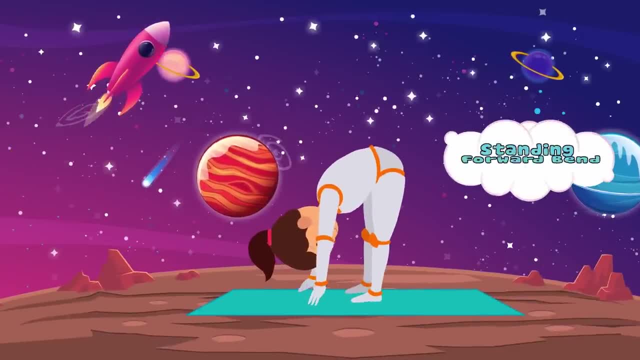 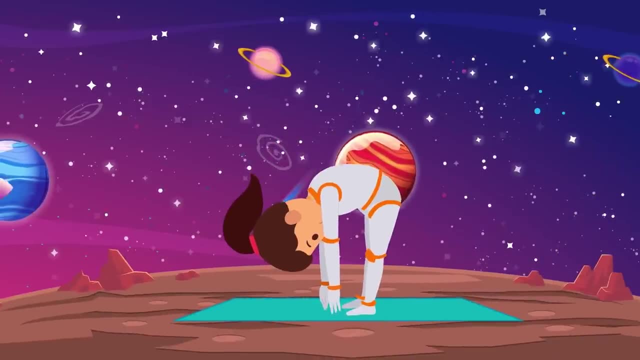 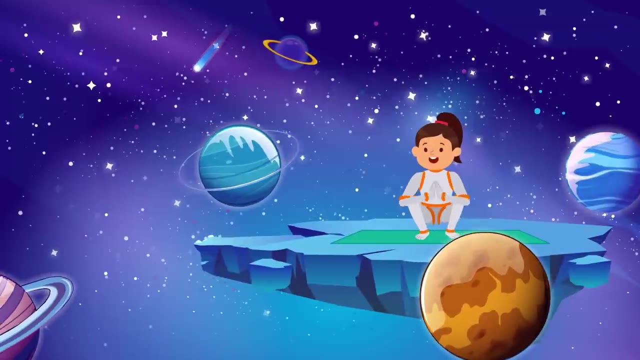 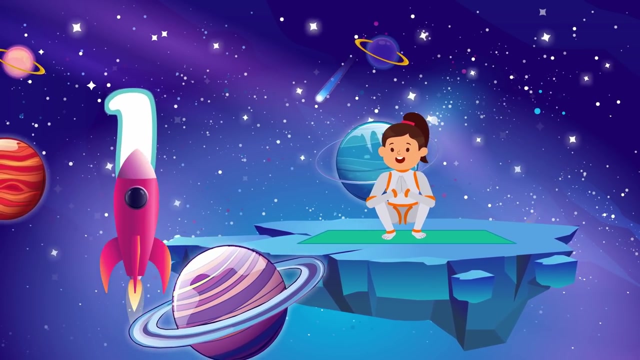 As my feet touch the ground, I explore what's around, Reach up to the sky where it's darkness- no light. Oh, let's get ready to go slow. Five, four, three, two, one, Blast off. come on everyone. 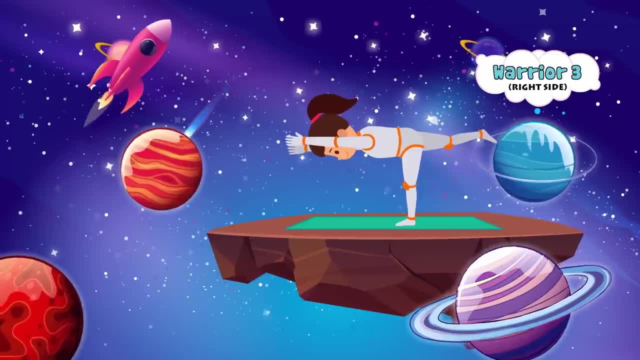 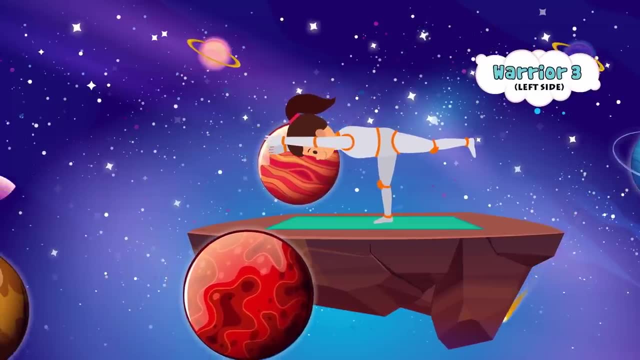 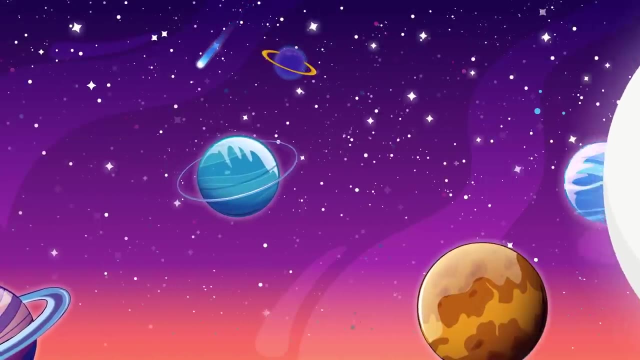 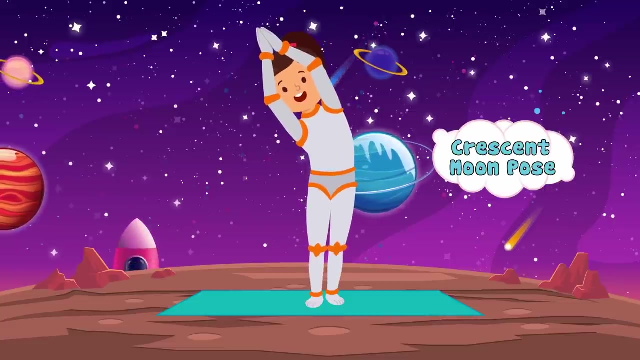 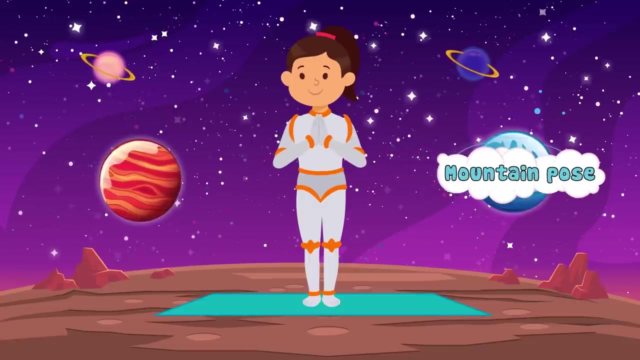 I like to take a rocket ship to the moon. Here's the part where we go: zoom. We fly out out to outer space. Fly out out to outer space. I touch one side of the moon and the other side too. I have come all this way on my own. I'm not heading home.